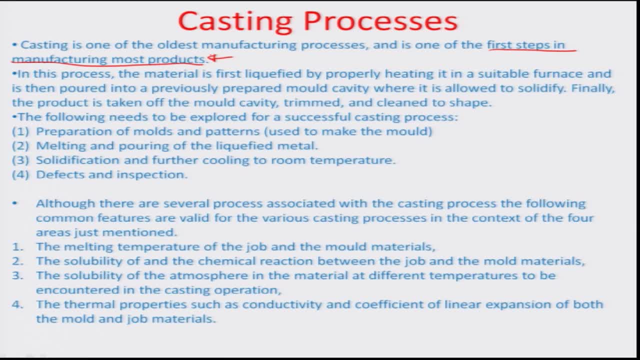 products to engineering assemblies by many secondary processes. So this is one of the primary processes of manufacturing. So in this process the material is first liquefied, as you know, by properly heating it in a suitable furnace, and then poured into a previously prepared mold cavity where it is allowed to solidify. So therefore, the 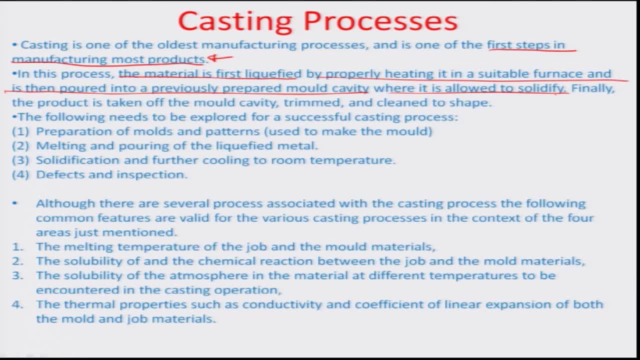 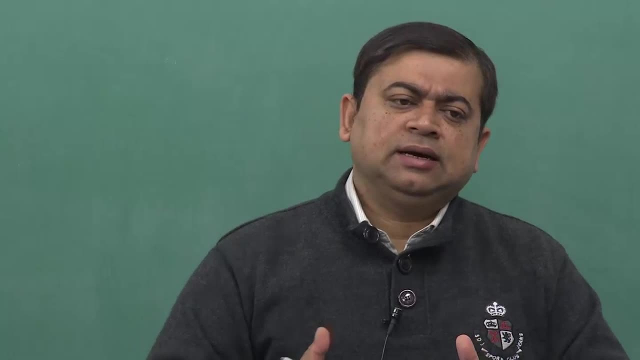 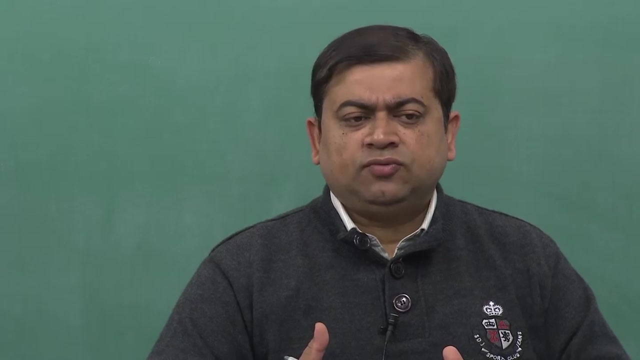 important aspect is that the liquid metal is first formulated and there is a question of liquid metal vis-a-vis liquid alloying, which happens because of the dissolution of a second phase in that, And then it is heated in a suitable furnace which actually takes, you know, its own, or it sort of imposes its own effects by the mode of heating, So for, 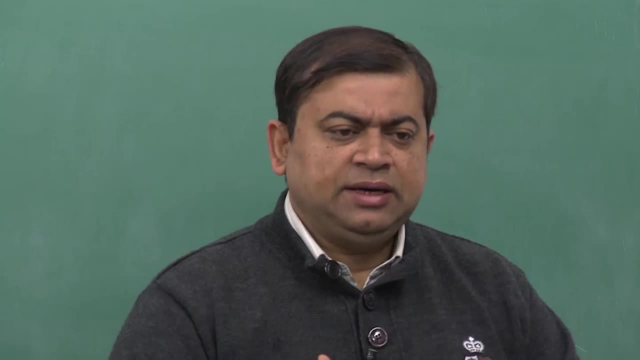 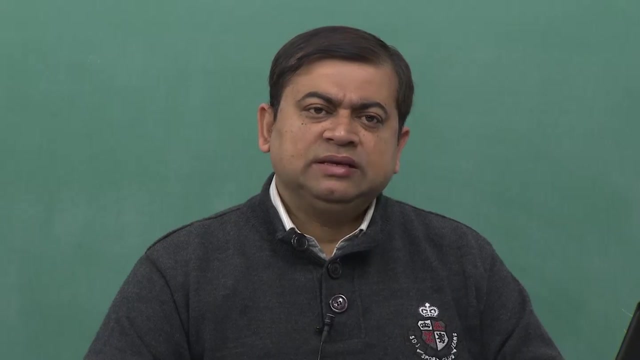 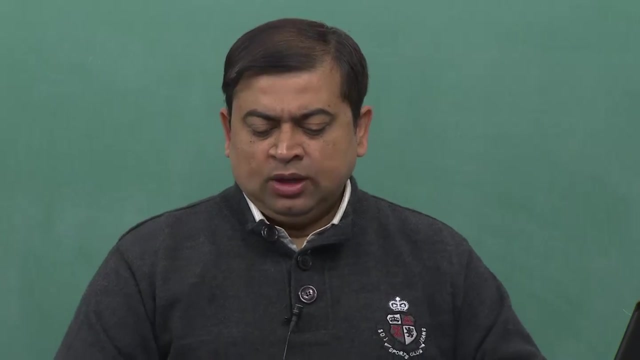 example, if the furnace is induction based, then the heating is completely homogenous throughout the material. but if a furnace is something where there is a- you know, wall based heating or the heating happens through the walls, there is going to be always temperature gradients which are going to be there. So when the product is finally taken off, then 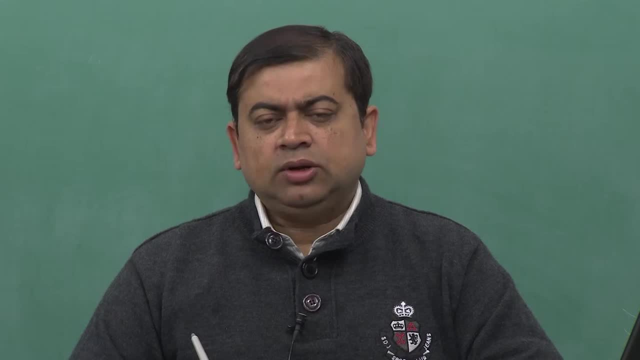 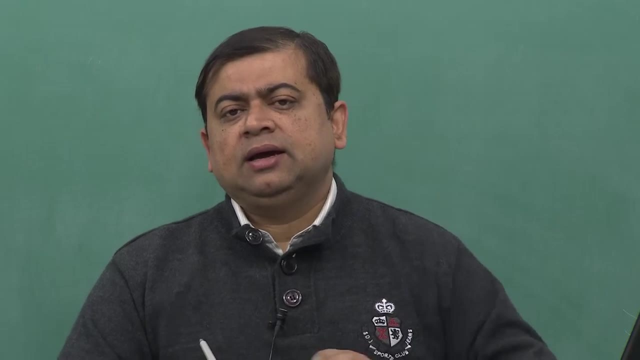 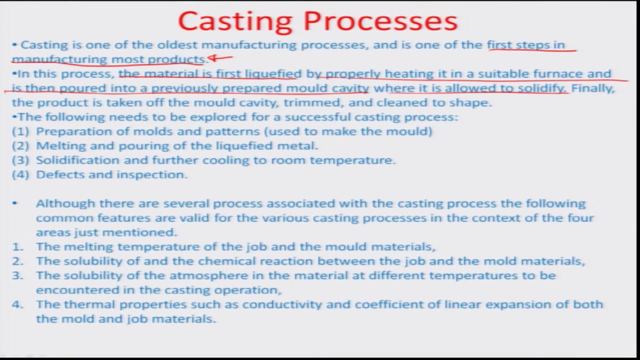 you can further process it, Trim it, you know, clean to the concerned shape, something you know which is more suitable for engineering assemblies, etcetera. And so the following needs to be explored for a successful casting process: One is the preparation of molds and patterns which are used to make. 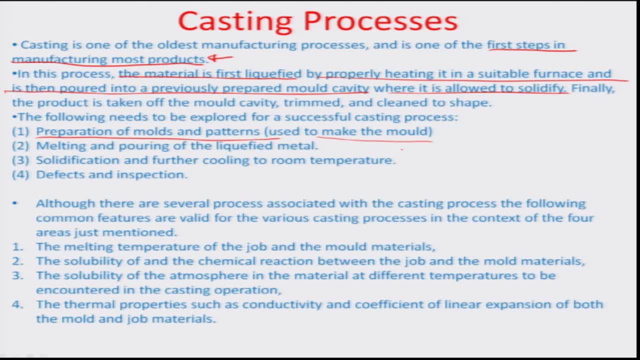 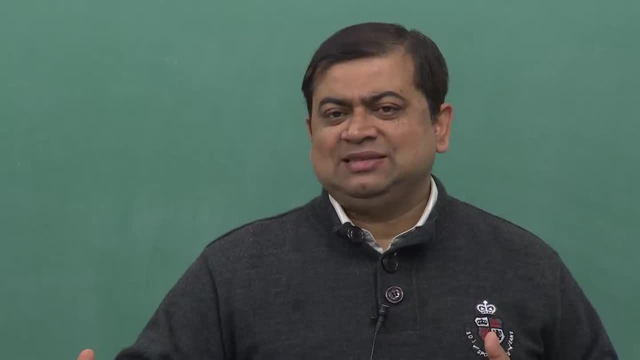 the mold. Mold basically is the housing which would hold the liquid metal till solidification. So therefore you need to be able to prepare it with the refractory material, normally sand molds, green sand molds are very commonly available because sand is a refractory material. 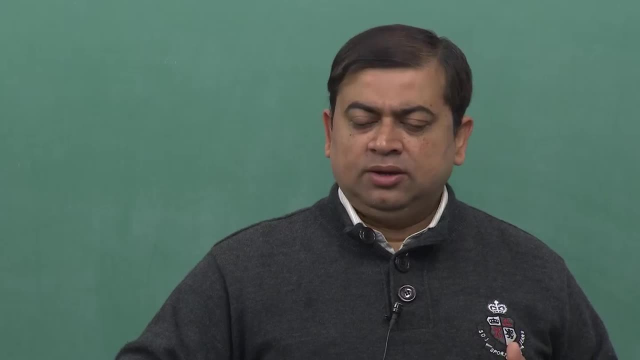 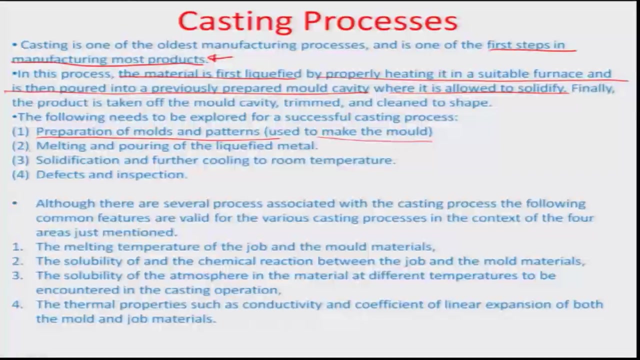 which can withstand high temperature and still be strong, you know. So that is why sand is mostly used. And then also you have to melt and pour the liquid metal. So there is a lot which sort of comes into way of this, because you are 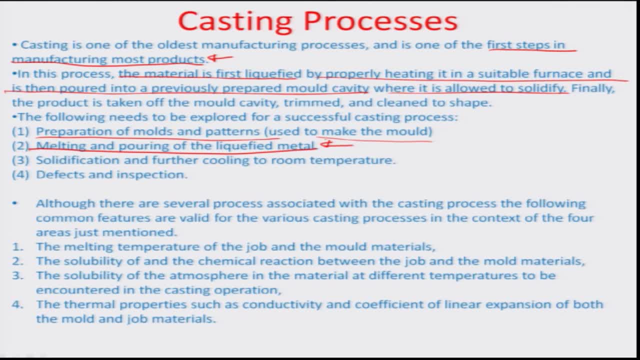 essentially passing it through a channel which is also known as the metal, the metal runner, and then there is a gate which goes or which throws off the metal into the cavity where the filling action starts taking place. And so, during all this process, there is always 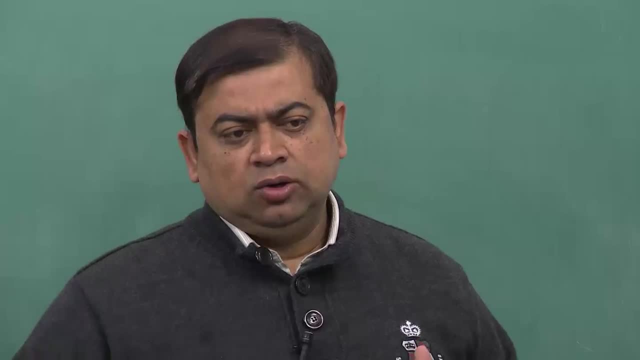 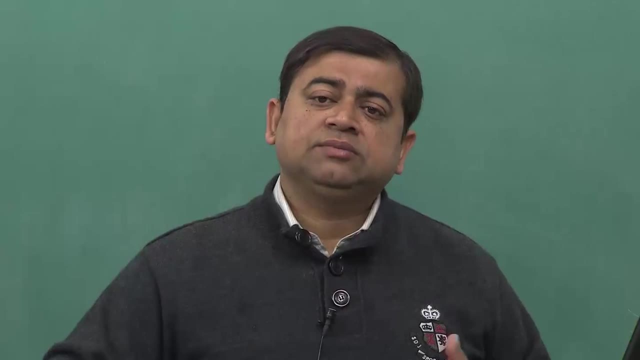 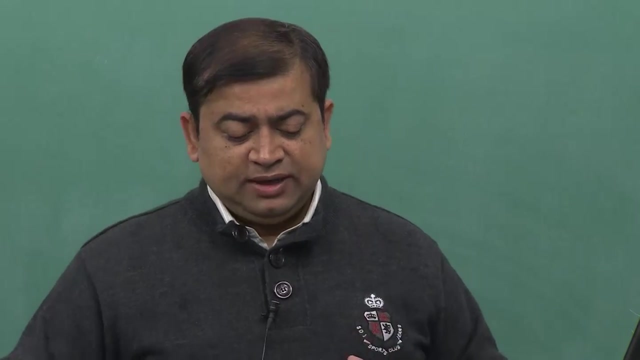 heat transfer because, remember, the mold is always at a lower temperature than the super hot liquid metal which is flowing through it, And therefore there is always a possibility of solidification before entering, And so the processes should be defined or designed in a manner So that liquid metal really enters before the solidification happens. 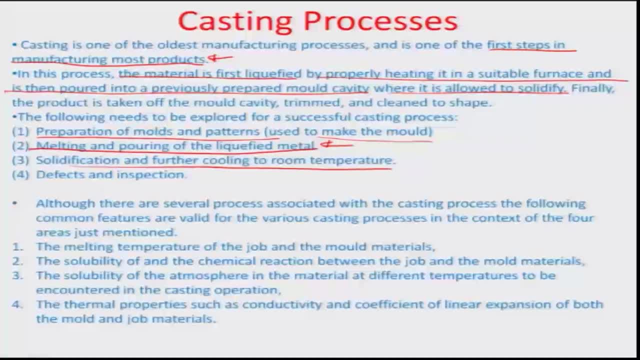 And then you have to give heat to finally the solidification and further cooling to room temperature. And one of the reasons why this is important is that you know we assume that most of the metal goes into the mold from the gate region as liquid metal And so once the liquid is now stationed inside, 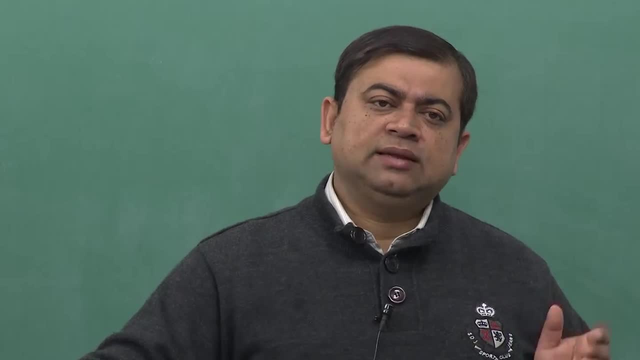 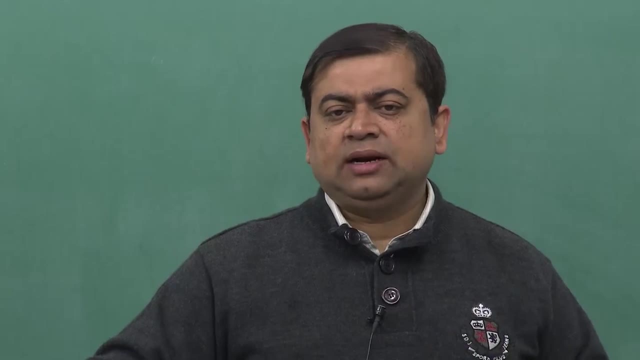 the mold and you have obtained the indication from the other side, which is also known as the riser side, that the metal has fully filled the cavity. There is going to be heat transfer of this metal to the casting walls, Pressure die casting where the metal is fully filled. 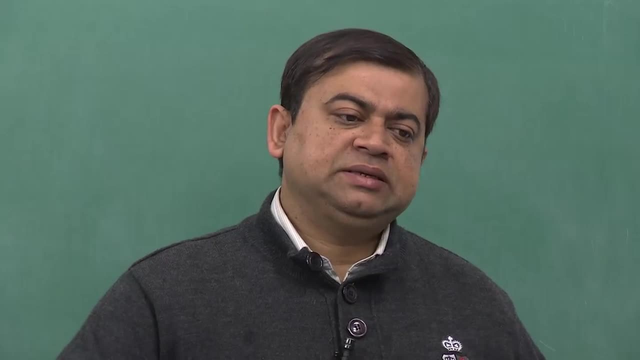 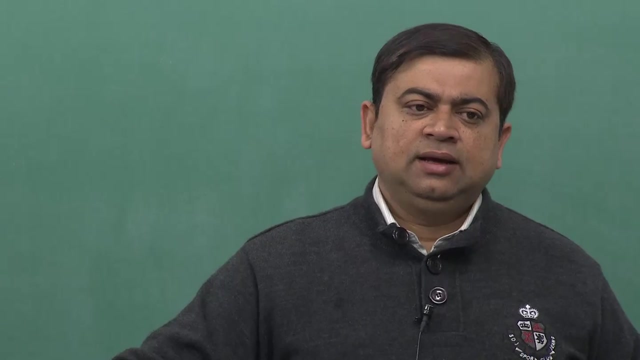 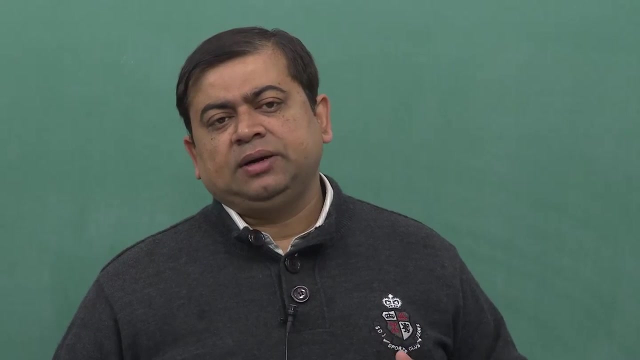 a metal mold is what is basically used for filling of the metal. So there the heat transfer rates would really define how the crystal growth would take place, And in fact that also defines what is the surface hardness of the casting vis-a-vis the hardness inside or even other many other properties like strength, overall ductility. 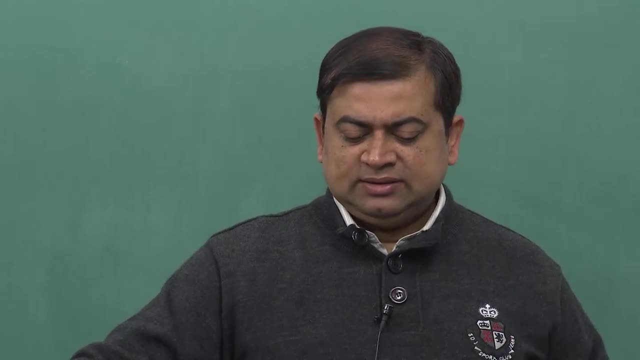 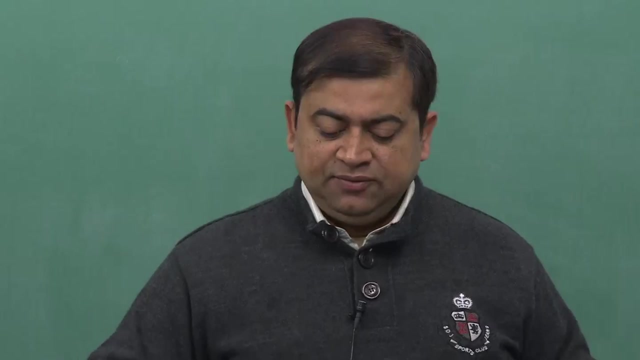 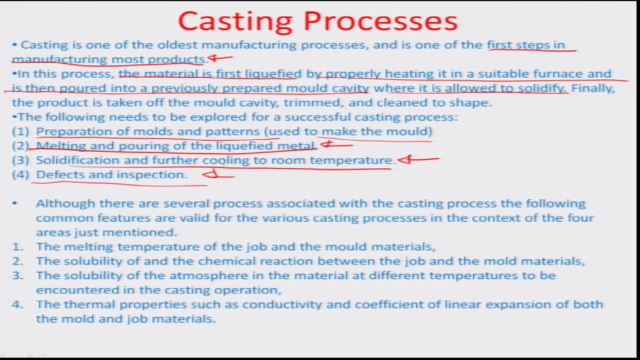 yield point, etcetera, related to the material casting. So therefore it is a very important aspect to become be considered while dealing with casting: solidification and cooling. So and then obviously, once the casting is prepared, then you have obviously it is not free of defect, So you have to have a method for defect inspection. 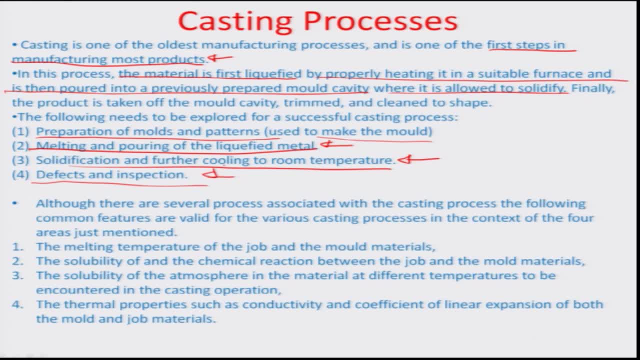 So you first understand some of the defects and then trying to inspect and remove, most of the time non-destructively, So that the casting material can be used for further processing. So, although there are several processes associated with casting, the following casting processes: 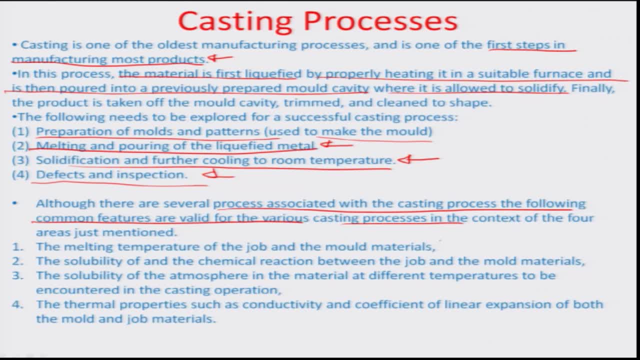 in context of the four areas just mentioned, One is the melting temperature of the job and the mold material. This is very critical because it should not happen that the mold starts melting away and joins the liquid metal because of the super heat that the material is in. So you have to be able to have a refractory in any event, which does not have its own contribution. 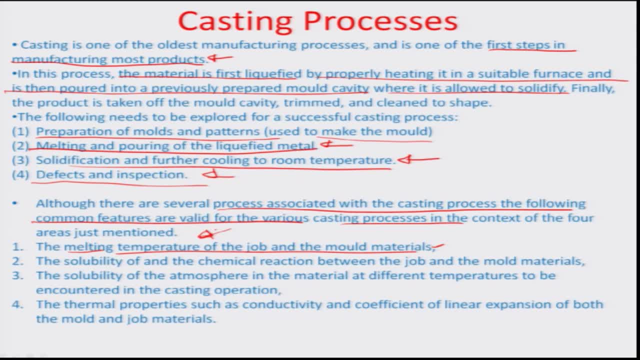 by melting into the cast. That is how the mold would be a mold material. The solubility of and the chemical reaction between the job and the mold materials also is a very critical aspect because obviously there is going to be out gassing, which happens. 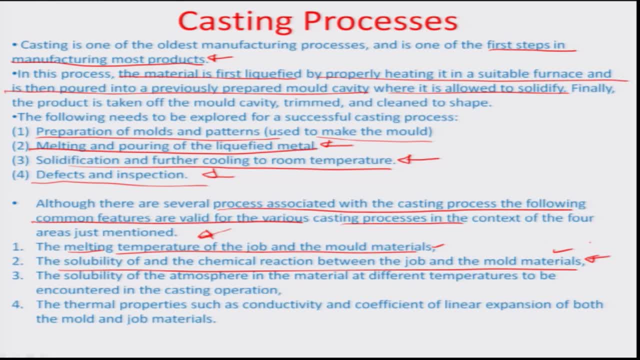 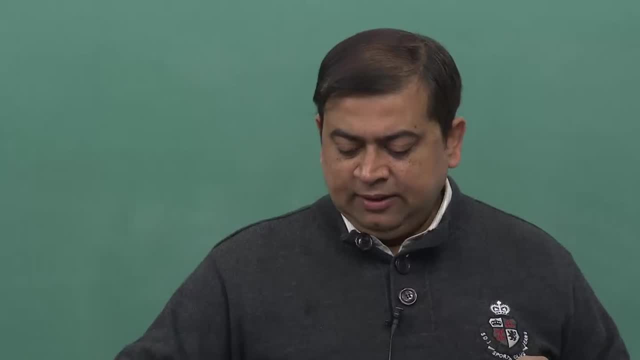 from the mold, or even at sometimes, if, supposing there is some organic which cannot withstand this high temperature, This can be entrapped as a vapor pocket within the casting material, and so in some cases, these may be very harmful because, primarily, it may react and make the casting very brittle Like hydrogen solubility is a major issue in castings because excess hydrogen may make the casting very brittle. So these are some of the issues. There should not be a chemical reaction which formulates a hydride or a nitride or a some kind of an oxide state which changes. 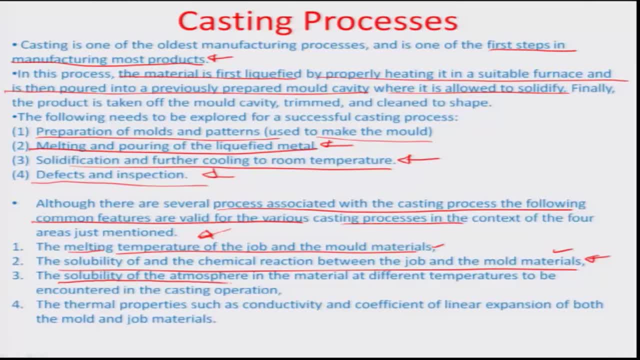 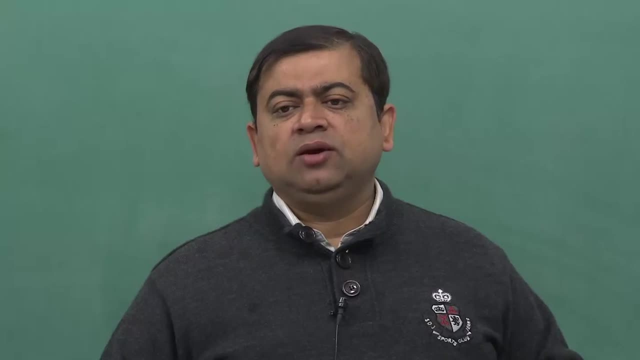 the property of the material. Obviously, the solubility of the atmosphere in the material at different temperatures to be encountered in the casting operation is also a major issue to be considered, because atmosphere itself has these gases and if there is a possibility of solubilizing the gases within the liquid metal, then it may mean a lot of property. 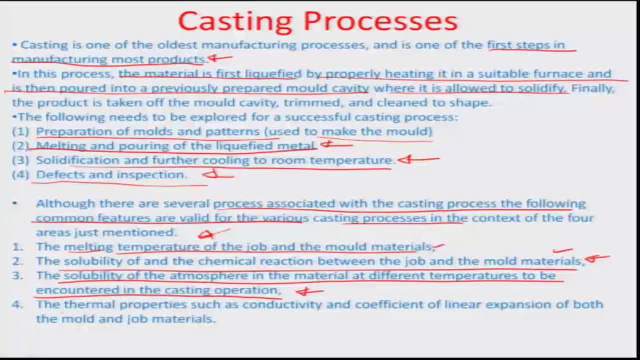 changes because of this solubility, The thermal properties, such as conductivity and coefficient of linear expansion, of both the mold and the job materials, which also are very important because you have to have an engineering dimension allocated to some material which is being cast. Therefore, you 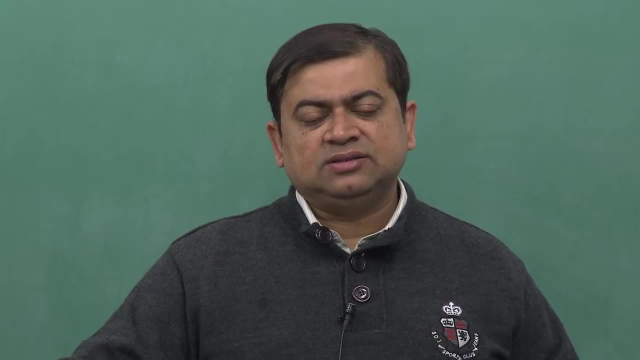 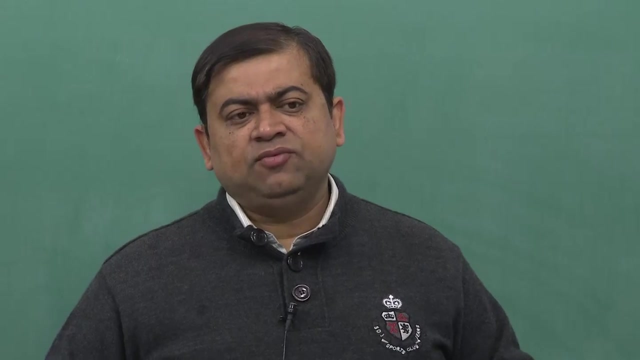 must consider allowances which are because of these shrinkage phenomenon. Obviously, metal poured in hot state is going toâm cool off, which is going to make the volume smaller, and then, obviously, it is also going to cool down further, from the solidification point to the room temperature, which is going 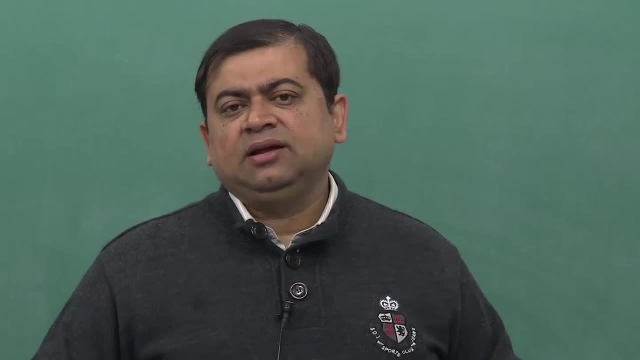 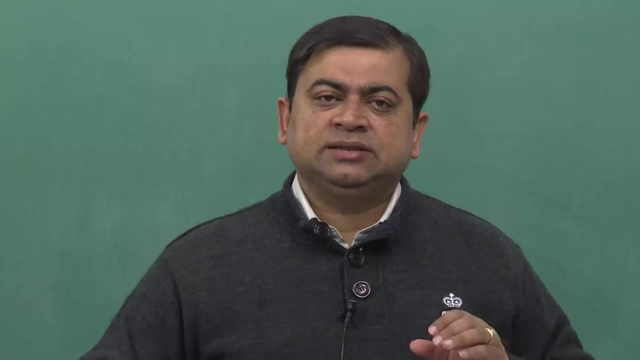 to be linearly contracting the material further. Therefore, you have to have sufficient allowances so that what you are getting is the final dimension, and the final dimension to be close to what the plant dimension is or the engineering dimension is of the particular casting. 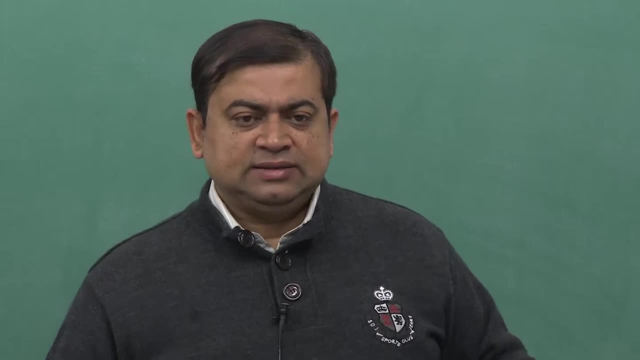 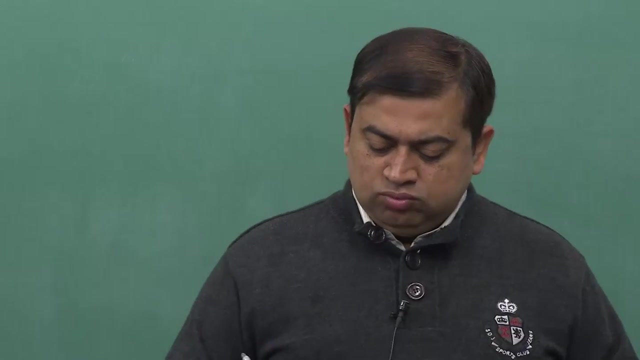 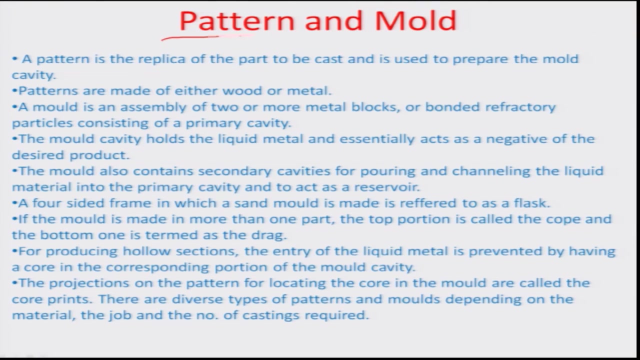 So you always need to give these allowances in the casting or in the mould design process so that ultimately, what you get is what you are looking for. So that is how you can say that castings can be sort of defined. So let us talk about now patterns and moulds. these are most important. pattern is something 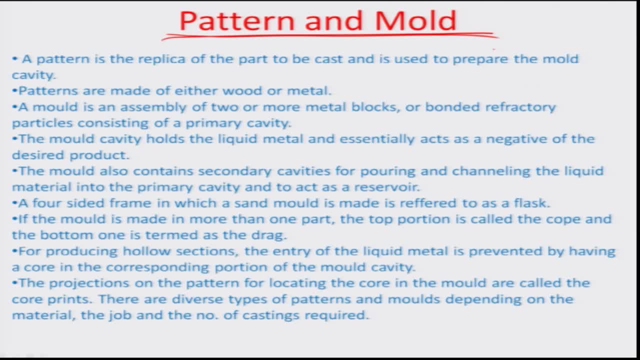 which is needed to formulate the mould. So a pattern is a replica of the part to be cast. it is used to prepare the mould cavity. So, obviously, if we are talking about moulds, So if we are talking about us, let us say: you know, sphere of metal, that we are going. 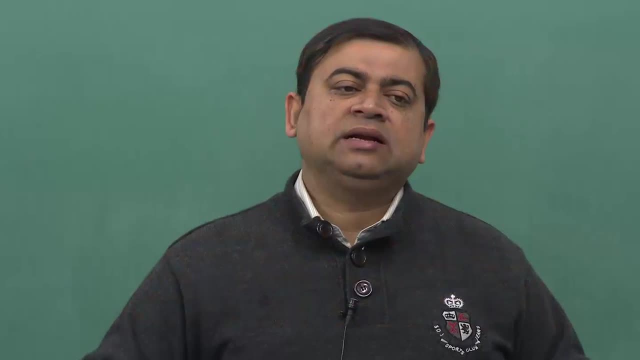 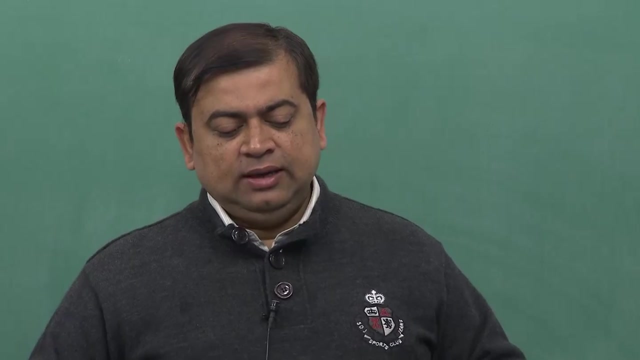 to roll out of a casting process. So the mould for that should be a spherical cavity into which the metal would go and then solidify and so be a sphere. So therefore, the pattern is exactly the replica of the parts and the mould is exactly. 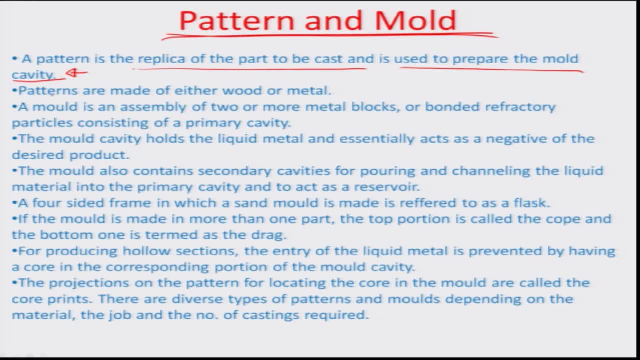 the negative of the part or the replica that we are talking about. So patterns can either be made of wood or metal. a mould is an assembly of two or more metal blocks, So obviously the mould contains the material which is used for making the mould cavity. 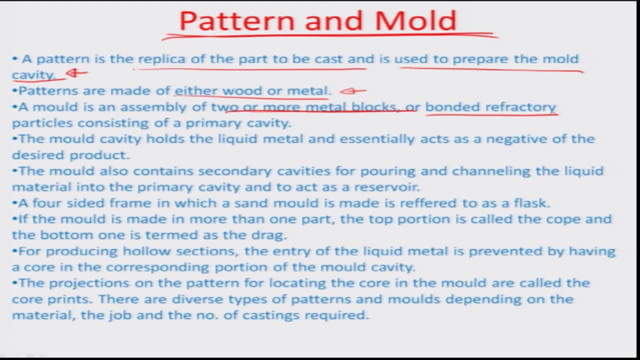 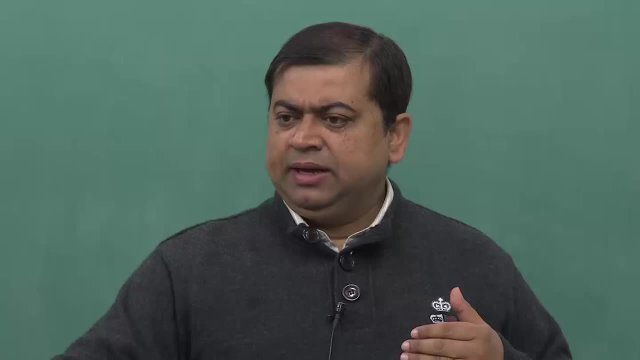 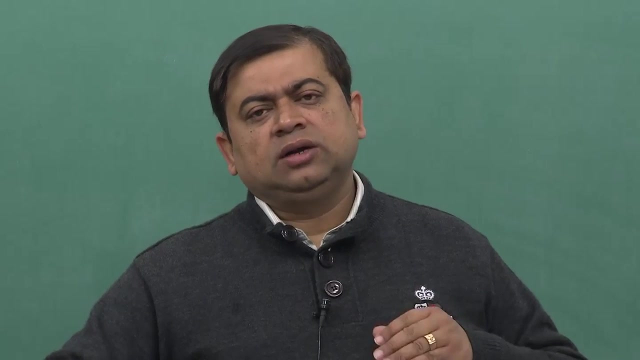 and this material is normally a bonded refractory which consists of the primary cavity where the metal should be filled, and the mould assembly. typically is made into two or more parts because you want to be able to pattern the mould and extract the pattern out. So actually the practice that is followed is that make a for a spherical pattern for. 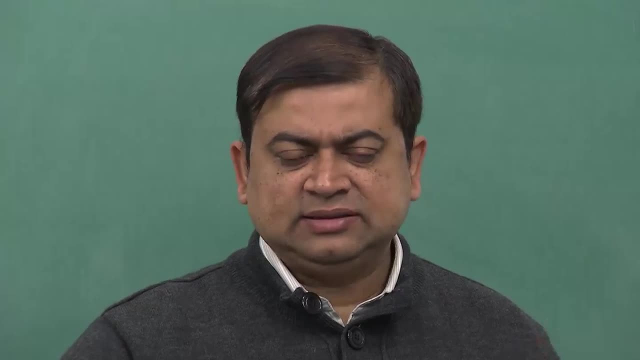 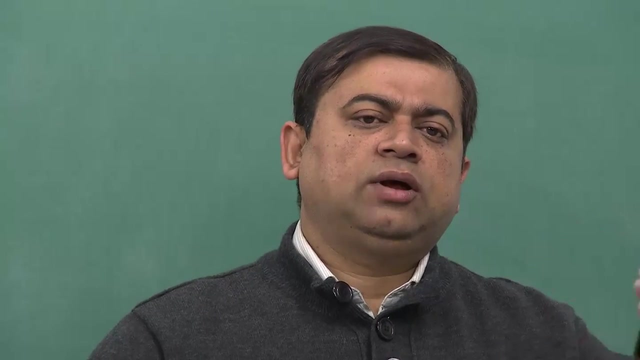 example, or you know, for a very large casting, let us say a casting of a wheel, you should have a half and half pattern, you know So. therefore, there is an upper half of the mould and the lower half of the mould. lower half is normally known as drag and the upper half is the cope, and then these two are actually 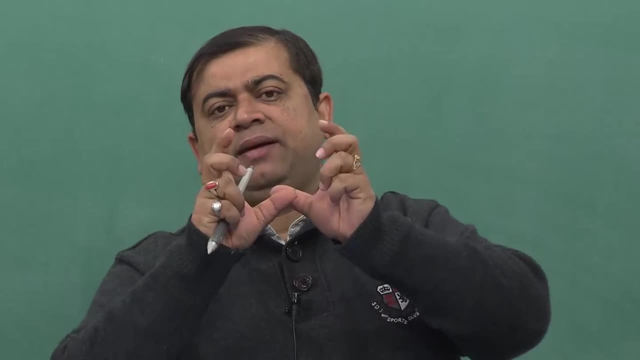 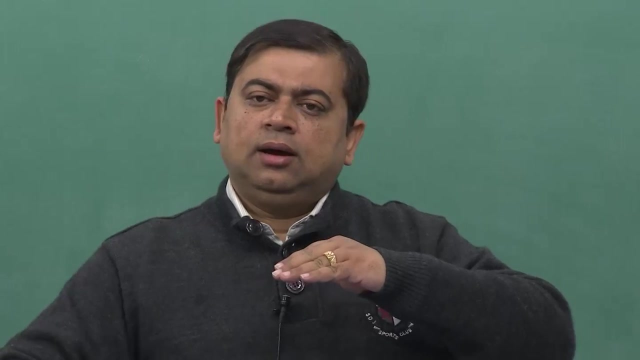 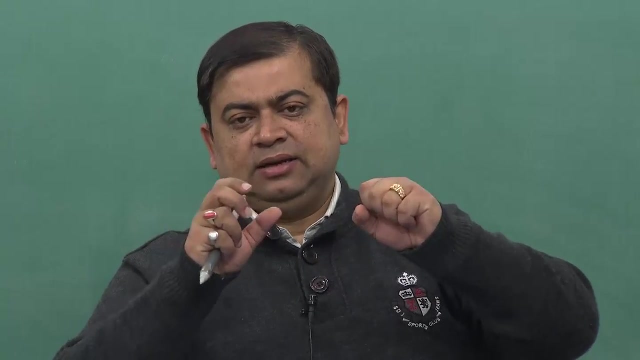 having a parting line, but the pattern is kept in a manner so that you have the split pattern, particular What we are talking about. you have half inside the lower portion and half the upper portion. So if we have, let us say, put this material inside the refractory material and before that, 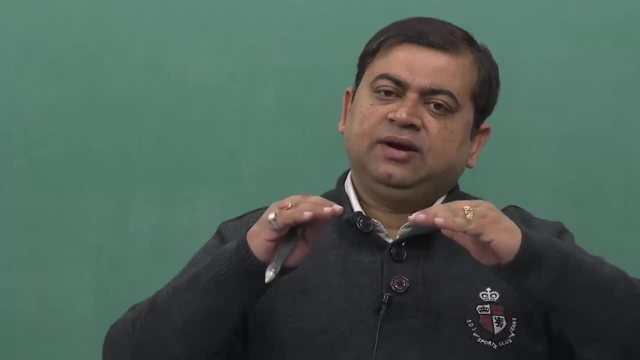 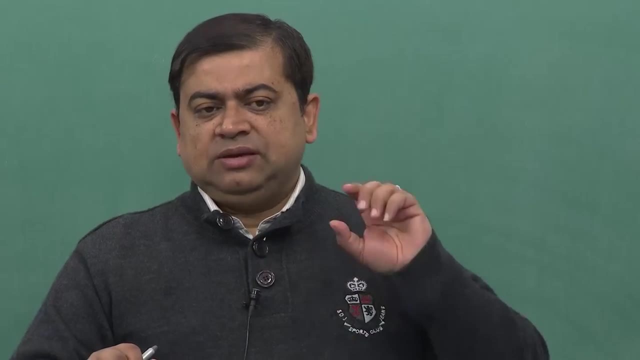 you have put the mould inside and then you have compressed the refractory material like sand and then you, when you remove the upper half and the lower half, you can extract the pattern away. and once the pattern is extracted and you close the upper half back over the 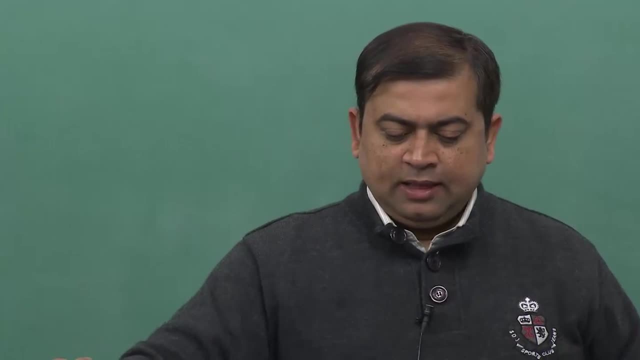 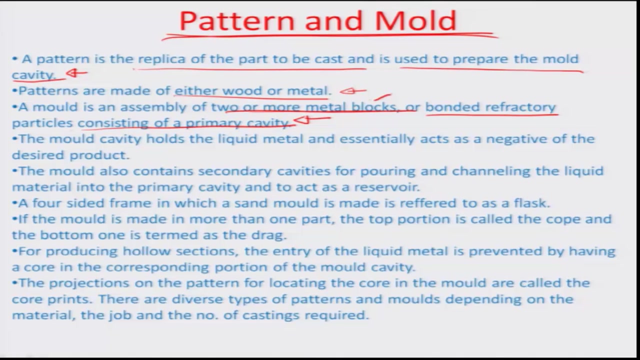 lower half. you have a cavity there. So that is how you basically. So that is how you basically making the mould. therefore, it is an assembly of two or more metal blocks, as has been rightly indicated here. The mould cavity holds the liquid metal and essentially acts as a negative of the desired 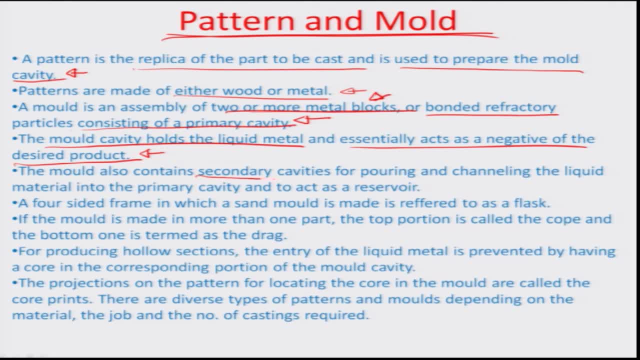 product. as I have already discussed, moulds also contains secondary cavities for pouring, channeling, etcetera of the liquid metal into the primary cavity, and this is, and also sometimes there is a cavity which acts as a reservoir for flowing the metal. So therefore you have the whole. 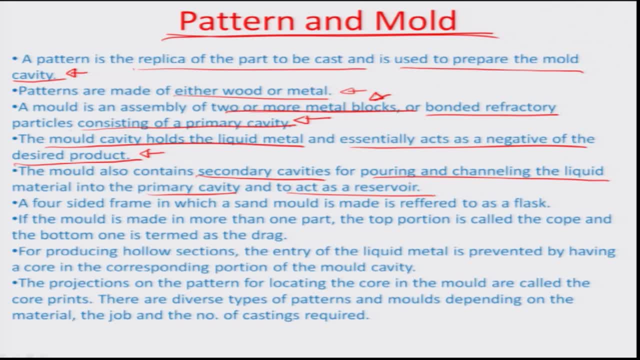 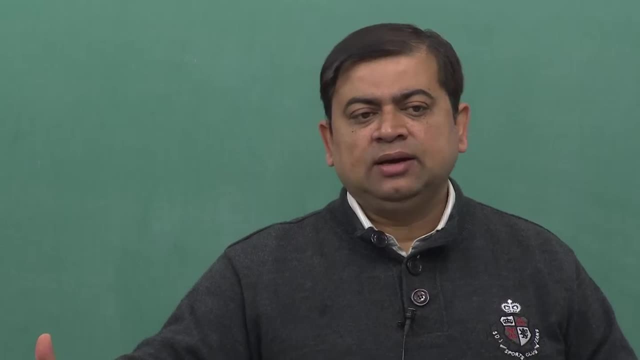 you know, pouring basin and then a runner and then a riser on the other side, which are cavities which otherwise would not be needed if there was no requirement of pouring the metal. So this is a sort of a metal channel, you can say liquid metal channel. 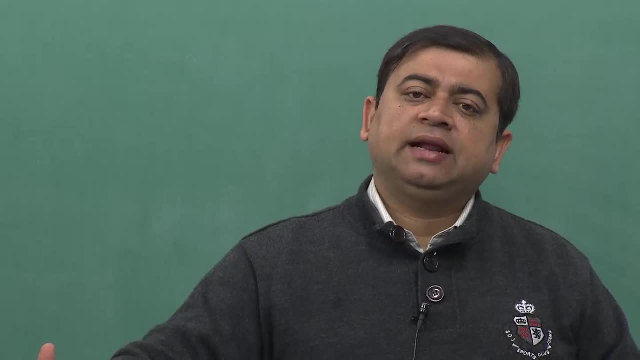 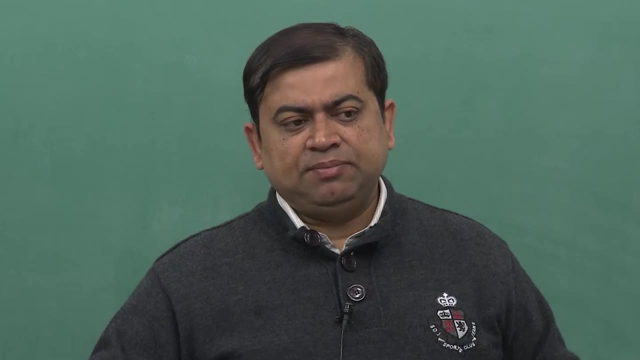 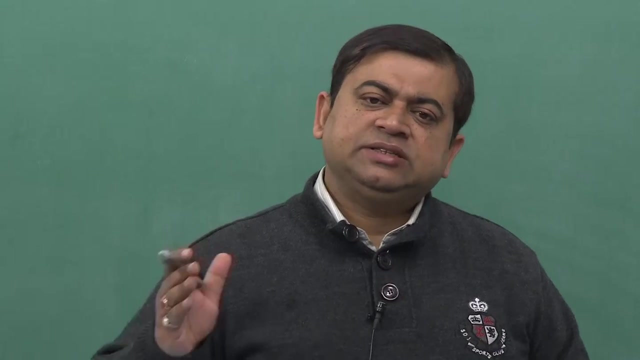 So this is also a secondary cavity. obviously this would get solidified and has to be removed once the metal piece is extracted, because the metal which is going to stay inside that cavity is also going to suffer heat loss and get solidified. So there is a trimming action which has to be performed on the casting almost always. 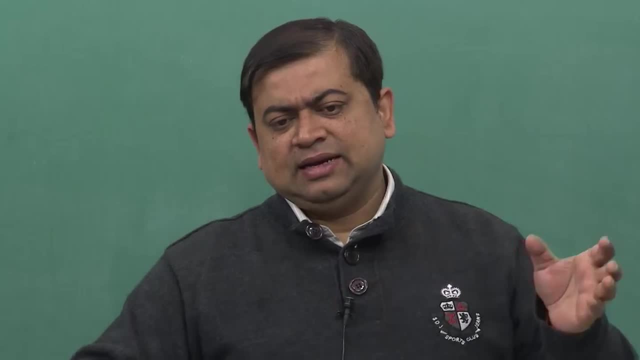 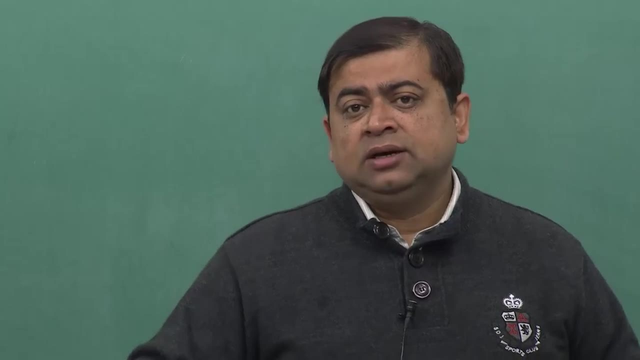 after extraction, So that these components or these parts, that is, the riser side or the runner side- has to be totally chopped off. you know, and that is how you recover the whole casting. So it is obviously a wastage of material because you want to design the riser and runner. 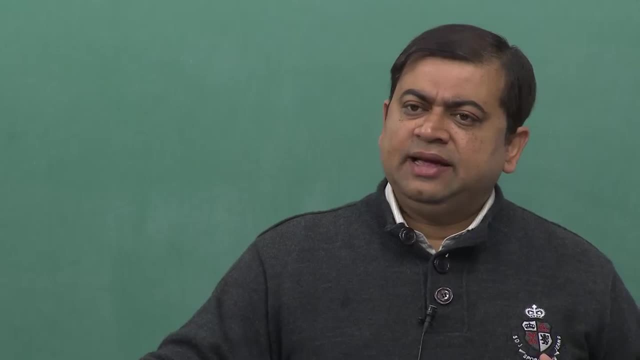 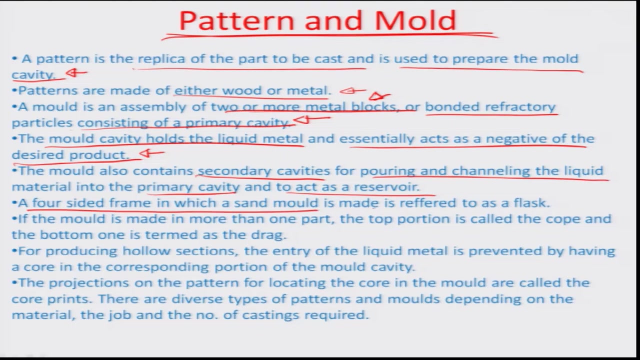 in a manner So that the wastage is Very little, but still there is going to be wastage of material during this pouring process. A four sided frame in which sand mould is made is referred to normally as a flask, So the mould is made of more than one part. the top portion is called the cope and the 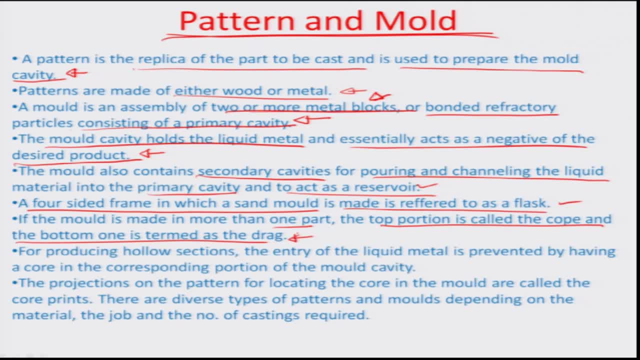 bottom one is termed as the drag, as I think I had already entered told you. And for production of hollow sections, the entry of the liquid metal is prevented by having a core in the corresponding portion of the mould cavity. So, supposing you wanted to make a 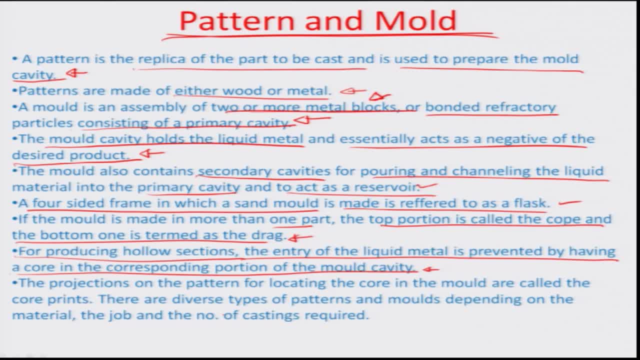 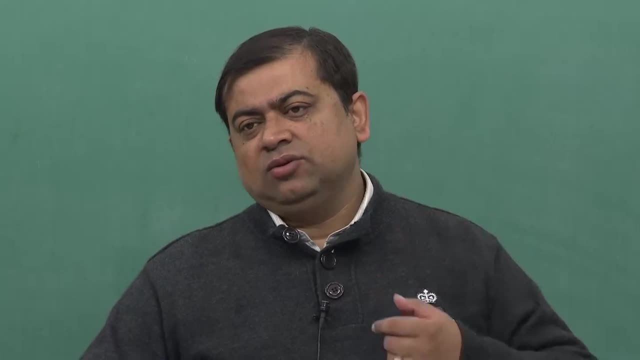 Hollow object. so obviously you would like that the metal does not go into that part of the mould where there needs to be a hollow. So you have to have something called a core and for supporting them you may have to need. you need some things which are like legs where the core can be standing on, which are known. 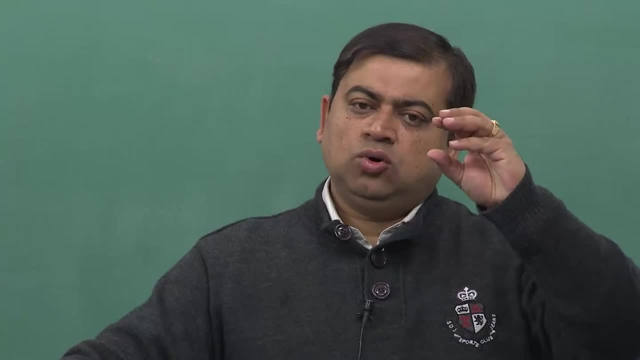 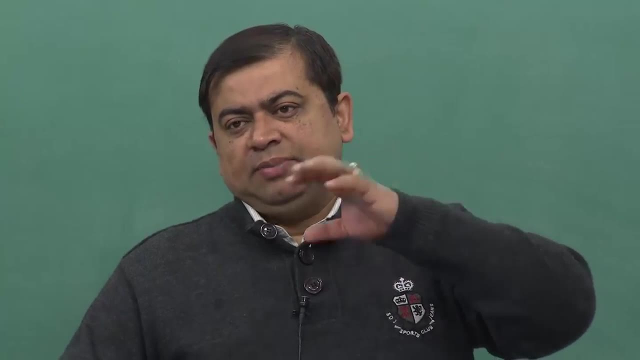 as core prints which are within the mould. So you have a small central core and some legs to hold that core in place, So that you know when the metal comes around it It basically Goes Around and you know it is not able to go into that region which has the core. 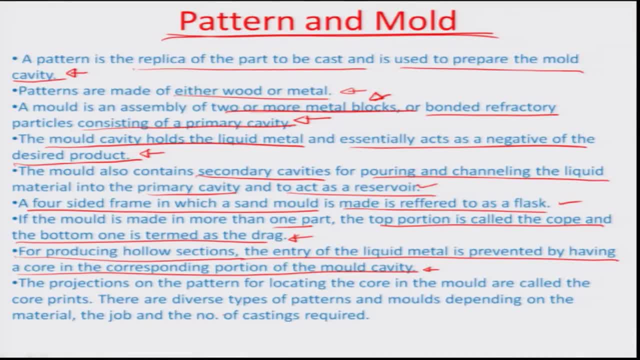 So you can exactly, you know, make the design in a manner so that the core can be extracted later on. So that is how you do this kind of hollow castings. so core is very important. The projection of the pattern for locating the core in the mould are called core prints. 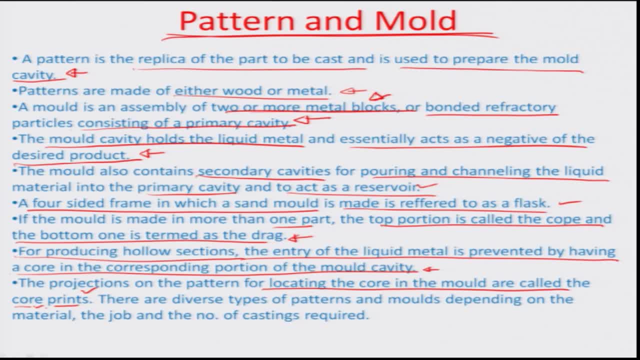 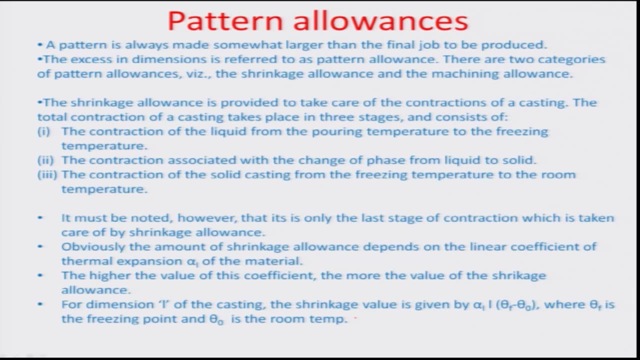 as I have just mentioned, it is like legs which are holding the core in place. there are diverse types of patterns and moulds depending on the material, the job and number of castings which are needed. And the first important consideration which one has for designing these patterns are pattern. 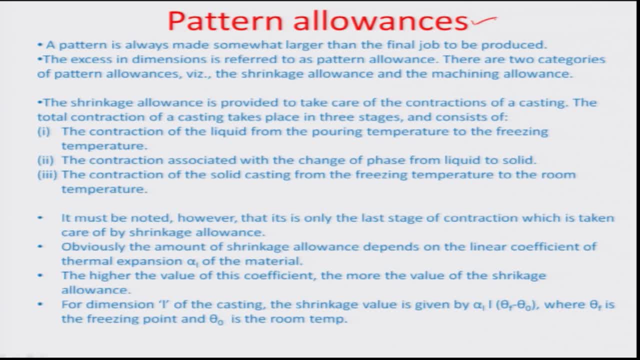 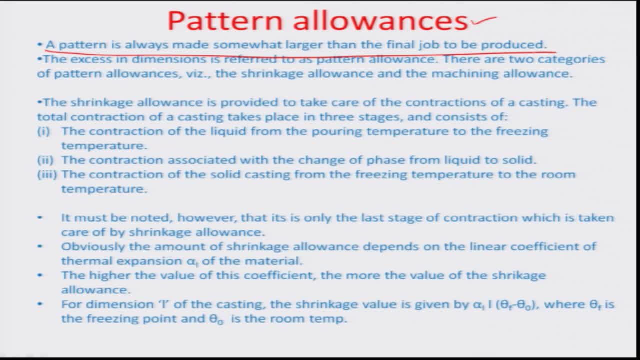 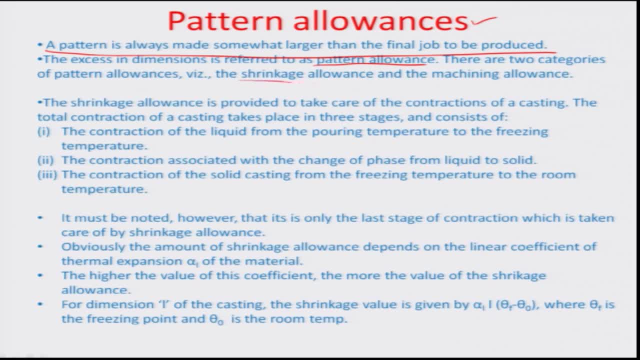 pattern allowances. There are two categories of pattern allowances: you have a shrinkage allowance and then you have a machining allowance. So, obviously, a shrinkage allowance, as I told, is more because of thermal issues associated with the sudden- you know, sudden- decrease in the temperature. 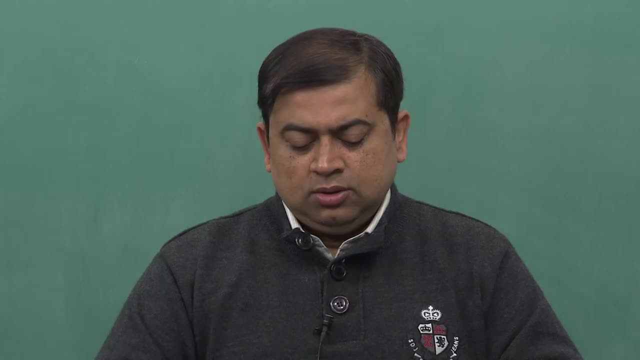 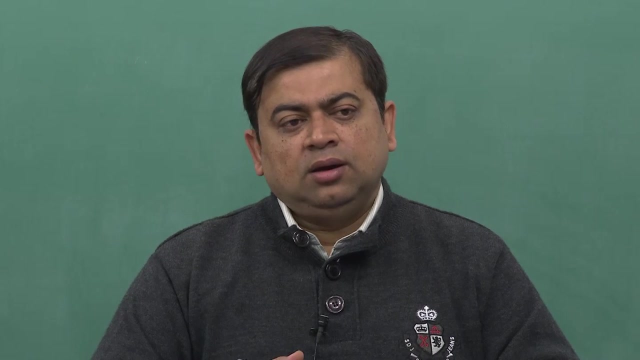 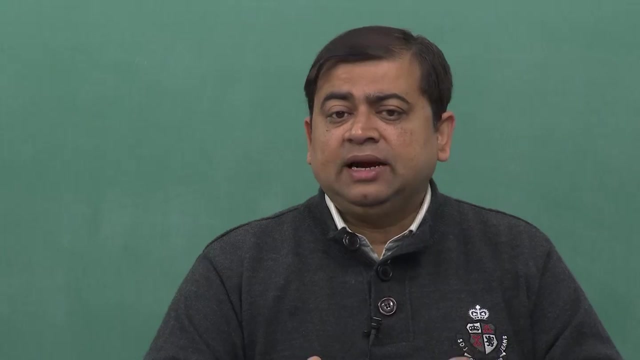 So the shrinkage allowance is a very important factor of the metallic system. But you know, ultimately this casting or this primary shape has to be fitted into an engineering assembly and it needs to be compatible with the tolerances or the overall you know, matching with that engineering assembly. 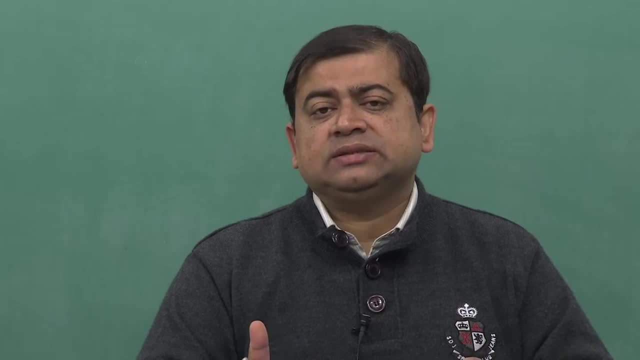 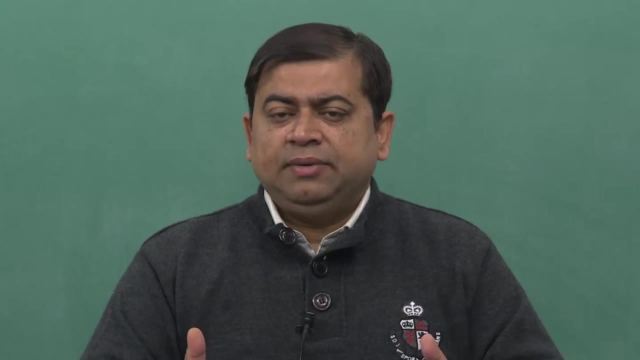 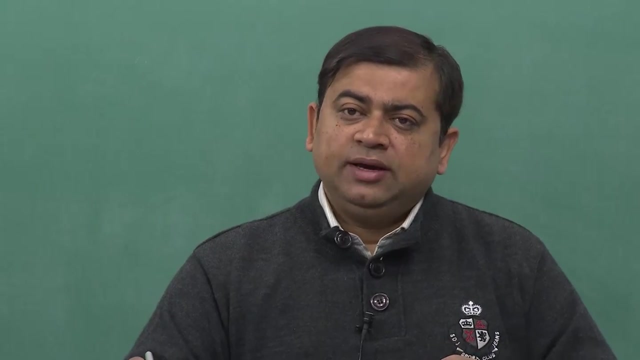 Supposing you are making a shaft, for example, and it has to fit into a certain hole, So there has to be some tolerances, you know, there has to be some fits of how the shaft is made with the particular hole in question, And so there are certain machining allowances which always need to be incorporated where 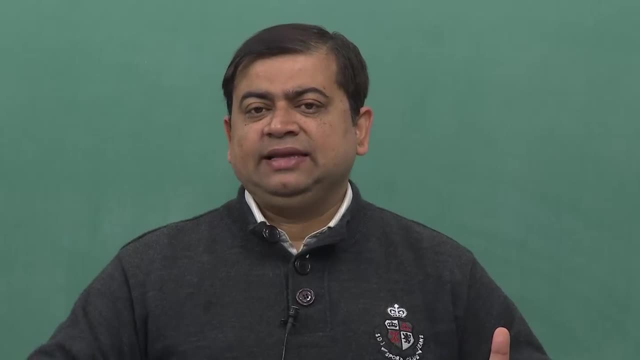 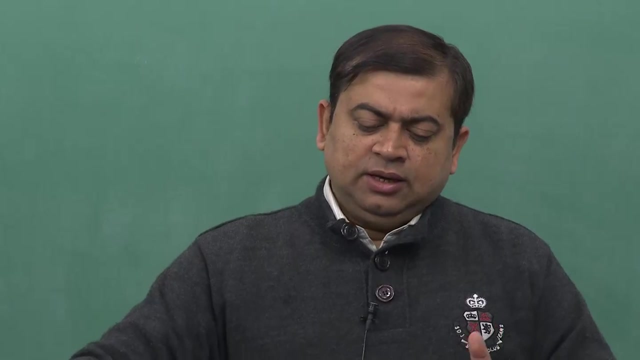 such fine machining operation on the casting would ensure that it has the exact dimensions and the tolerances that are needed for that casting to participate into a assembly, an engineering assembly. So there is a shrinkage allowance because of the metallic, the property of metals to 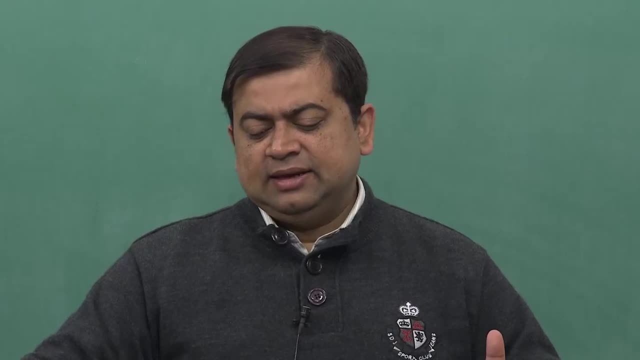 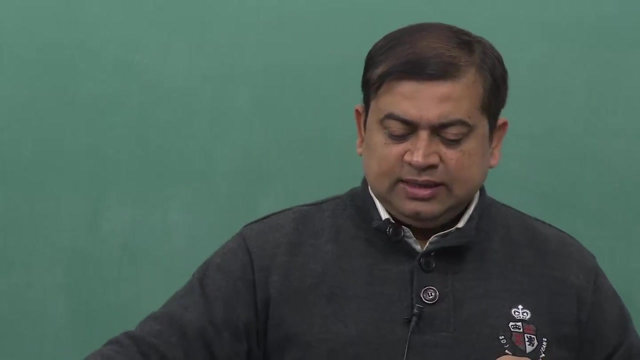 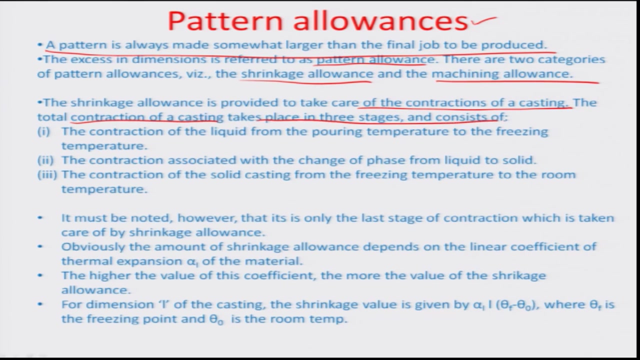 contract when temperature goes down. and then there is a machining allowance Which is used, useful because you want to fit these into assemblies. So the shrinkage allowance is provided to take care of contraction of a casting. as I told you, the total contraction of a casting takes place in three stages. one is the contraction. 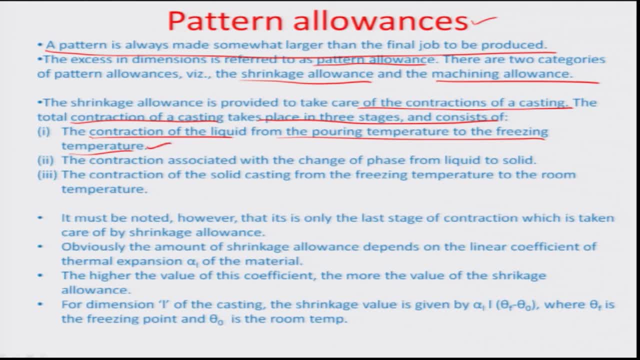 of the liquid from the pouring temperature to the freezing temperature. You have to understand, the pouring temperature is way above the freezing temperature And so, therefore, there is going to be some kind of contraction of this liquid. there is going to be a contraction associated. 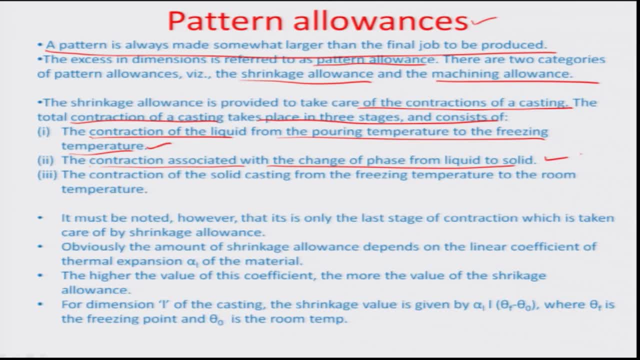 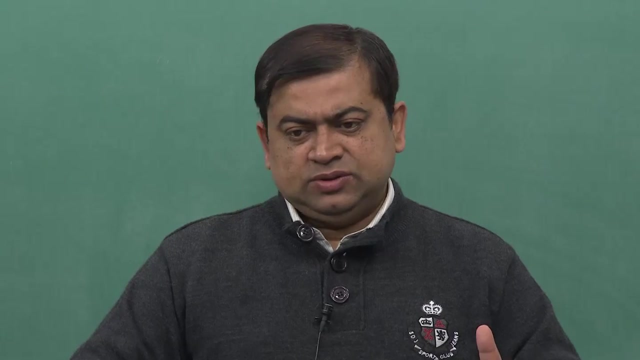 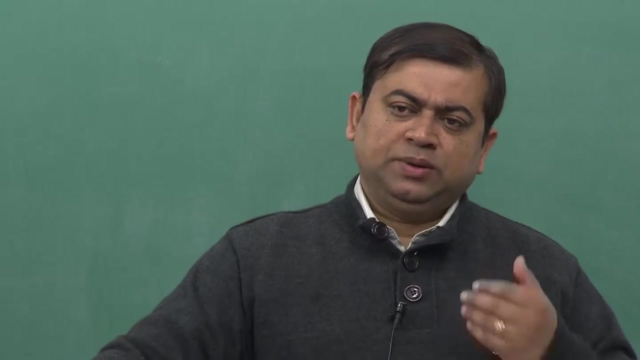 It may be possible that you superheat the material, and the pouring temperature and freezing temperatures are way apart. because of that and because of some reasons- because you want the metal to be transported in longer runners or longer risers- you do this intentionally, that you superheat the material above the liquefaction point, you know, or the let us. 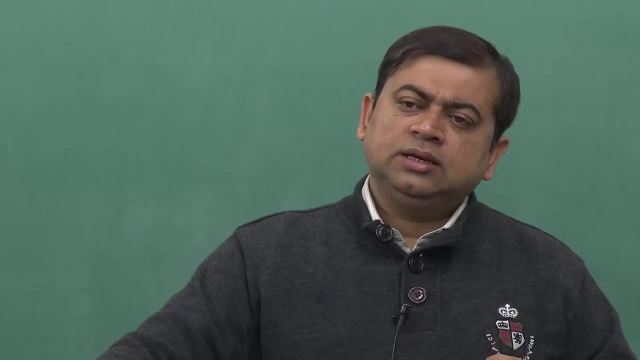 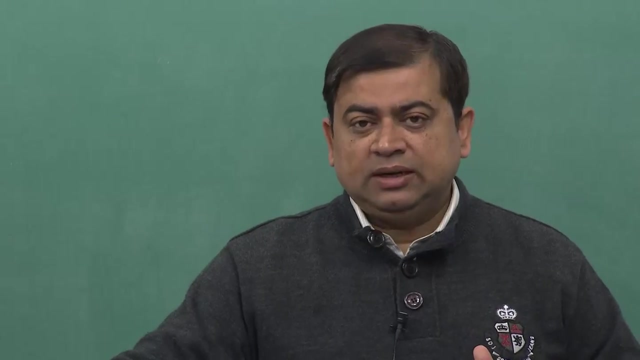 say, the freezing point. So there is going to be a difference in temperature there and so that when this temperature changes, obviously there is going to be a change in the overall volume. So this is very important: the overall volume of the metal which is in question. 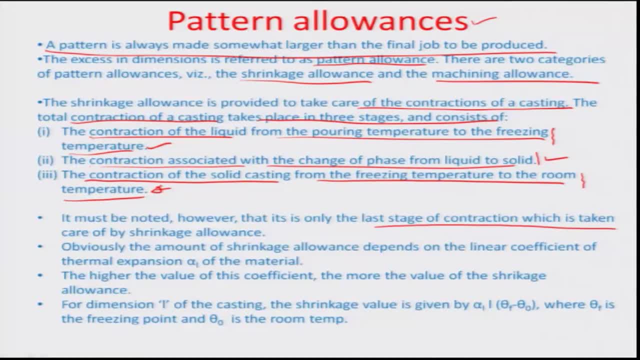 So it must be noted, however, that it is only the last stage of contraction which is taken care by the shrinkage allowance, because these two stages, that is, the liquid contraction and the change from liquid to solid, the contraction is very, very minor, you know, and that need. 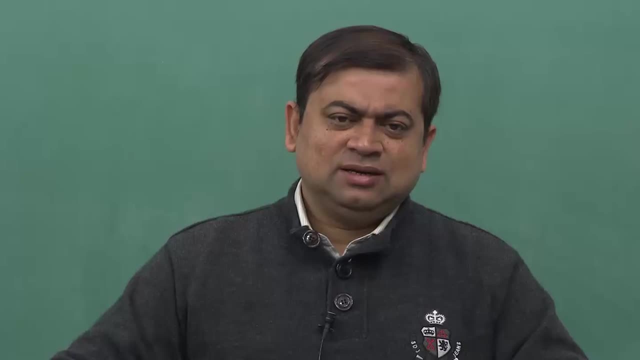 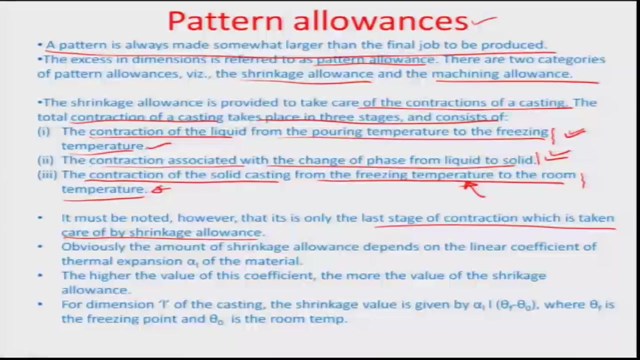 not be considered And probably some of these always gets cleared off because of machining and other processes which follow the casting process. So obviously the amount of shrinkage allowance depend on the linear coefficient of the thermal expansion of the solid material, that is alpha. 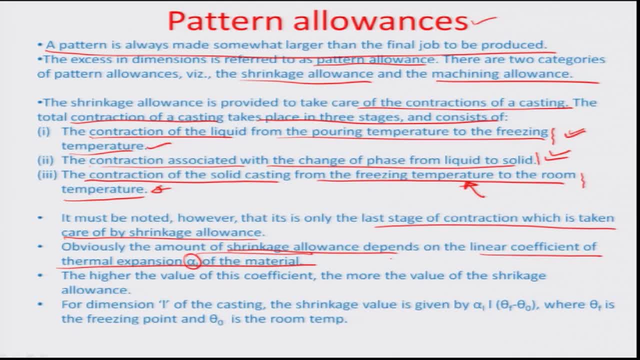 L. Once the freezing has happened, the shrinkage always, the major shrinkage always, takes place after that freezing process. So the higher the value of this coefficient, so higher is alpha, the more is the value of the shrinkage allowance and for dimensions L of the casting. 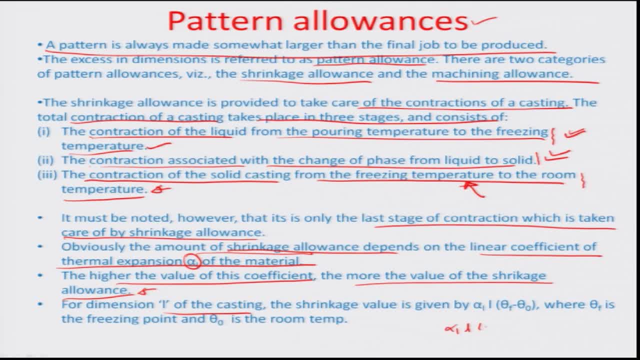 let us say the shrinkage value is given by alpha L, times of L, times of theta F minus theta 0, where theta F is the freezing temperature at which the material starts to solidify, theta 0 obviously is the temperature which is the room temperature. So obviously, when the 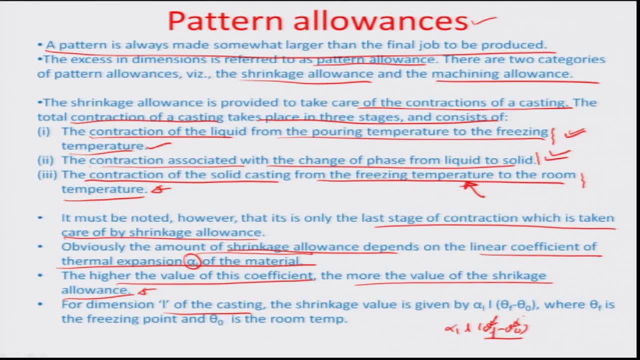 metal has just frozen to still hot and frozen to solid and from there slowly there is cooling to the room temperature. So the amount of delta L and the change in length which happens is actually proportional to the original length and is also proportional to the difference. 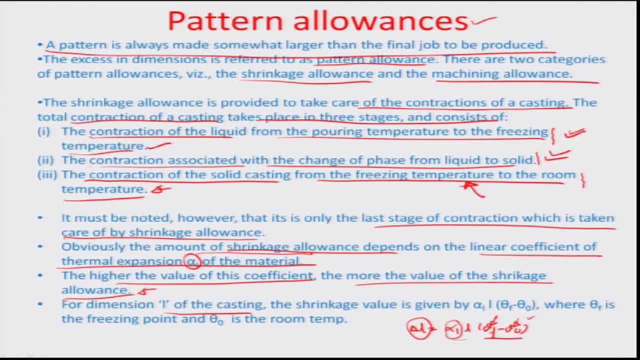 of this temperatures, and obviously alpha. L then is a thermal coefficient, a thermal expansivity coefficient which has to be proportional to the original length. It is a constant for a particular material system. So the shrinkage value normally which is given to the casting are, you know, recorded here, For example in cast iron shrinkage. 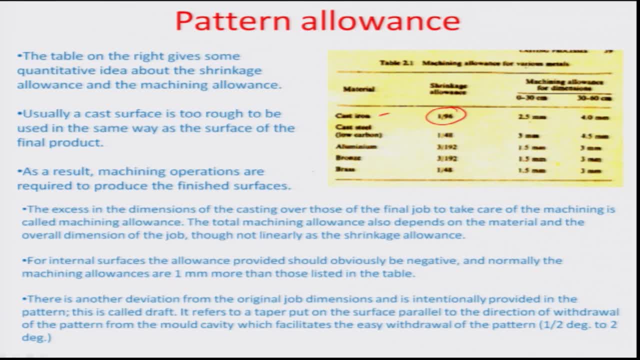 allowance is typically 196, and you know, for if you look at the machining allowance side, for dimension 0 to 37, you give machining allowance of 2.5 mm. So these are some thumb rules which people have generated who have been running these casting industries. If you have machining, 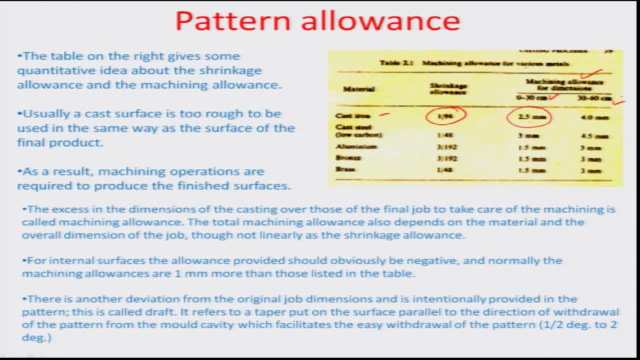 allowance 30 to 60 centimeters, the you know, for a dimensions 30 to 60 centimeters, the machining allowance would be about 4 mm, so on, so forth. So, similarly, you have cast steel, low carbon, which has a shrinkage allowance 148th of the actual dimension, which is in. 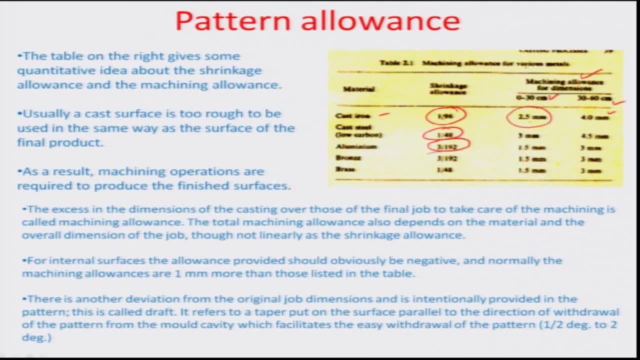 question: aluminum, which is 3192, 3 by 192, bronze 3 by 192 again, and brass, 1 by 48 again. and then the machining allowance for the dimensions are given here as 3 mm, 1.5 mm. Similarly, for 30 to 60 cm dimensions the machining allowance is 4.5 mm or 3 mm for cast iron, cast steel.